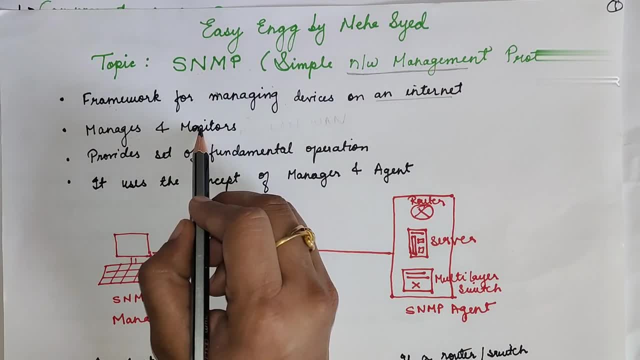 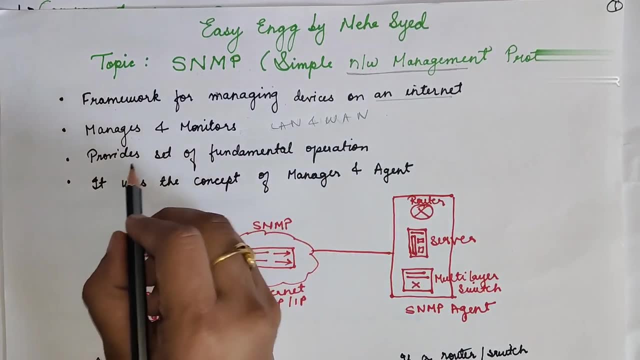 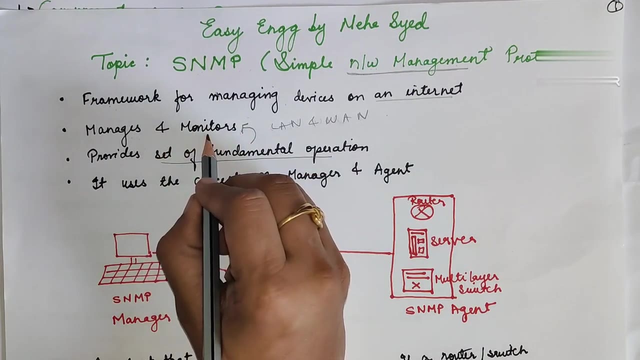 only managing, but it is also used for monitoring the network devices on the LAN and WAN. It provides the basic set of fundamental operations so that it can easily manage the network or monitors the network. So it provides the set of operations for it managing and for monitoring the. 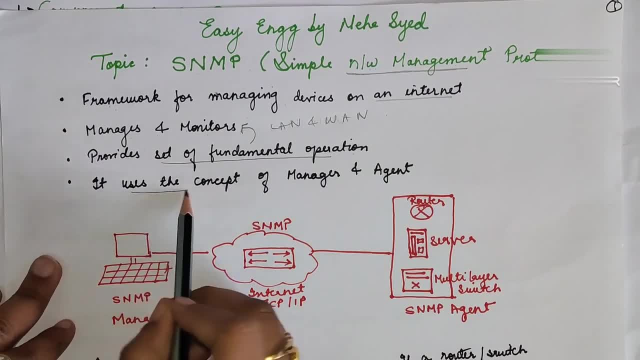 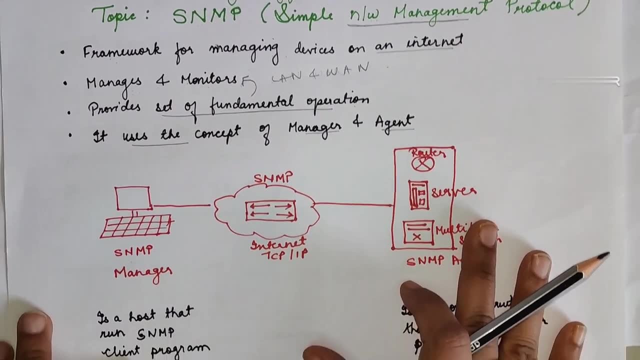 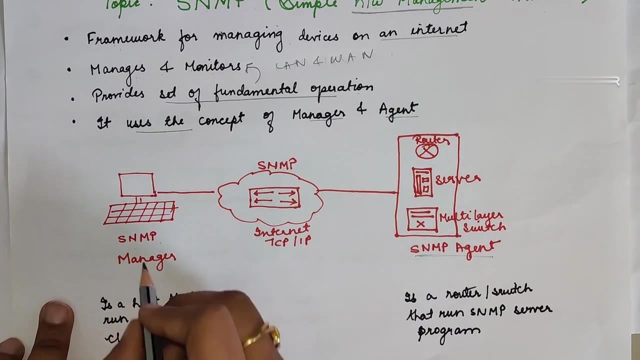 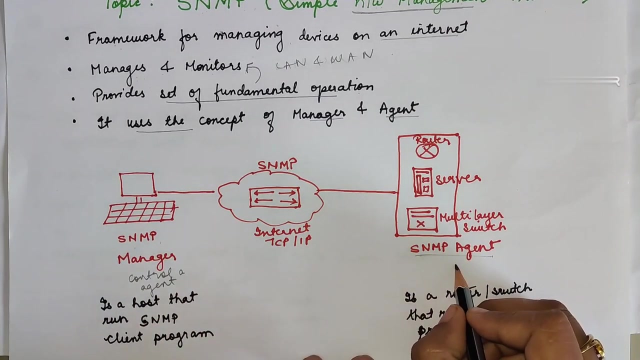 network devices And it uses the concept of manager and agent. There is one manager that we call it as an SNMP manager and another is an SNMP agent. So what is this SNMP manager? It actually controls the agent, whereas SNMP agent? you can say that it is a collection of different component. 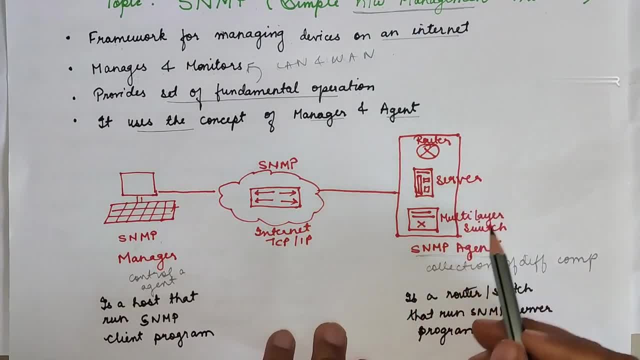 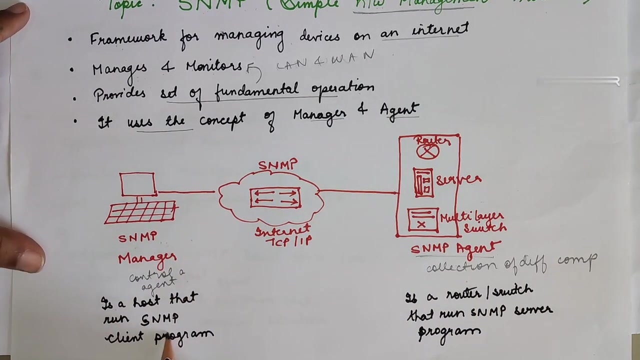 What are these different components? It can be router, server or the multi-layer switch. The different components. you can say that it is used for managing the network. So SNMP agent is a collection of different components and SNMP manager- it controls this agent. Now, one more thing you have to remember is it is a host that actually going to run the SNMP client program, whereas it is a server. 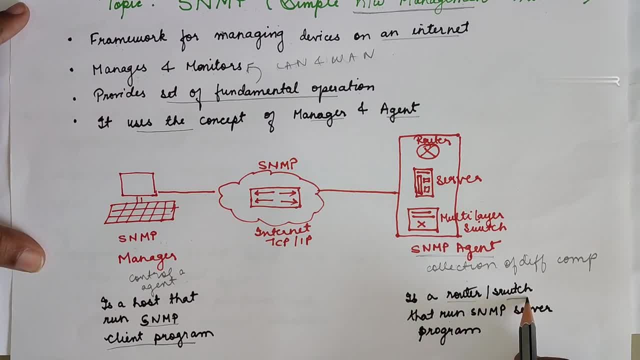 which actually you can say that there can be routers, switches or the server that are going to run SNMP server program. So the client sends the request. you can say that SNMP manager sends the request to check the SNMP agent. is there any fault in the network or is there any kind of congestion, for example? 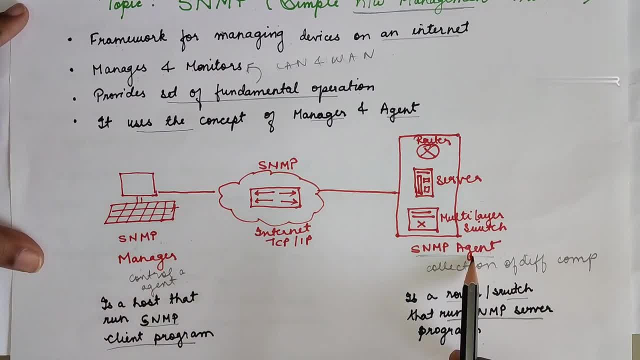 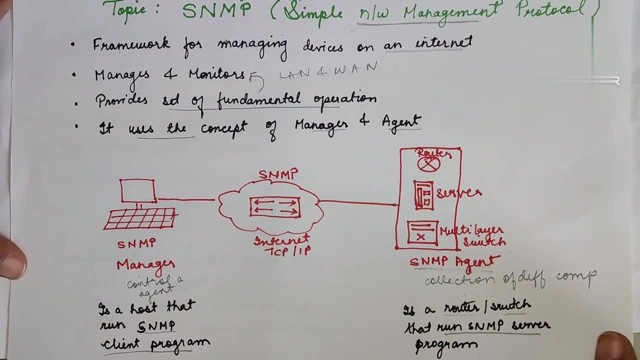 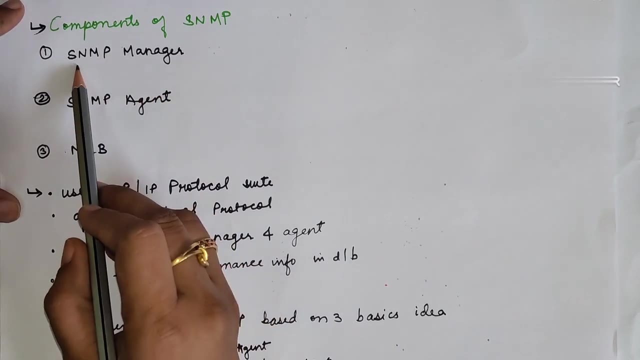 So it manages with the help of the manager and agent. So it manages the network very easily with these two components. Now one more important thing that I am going to show: What are the different components of SNMP? Let's go through once again: SNMP manager, SNMP agent and one more important component is an MIB. 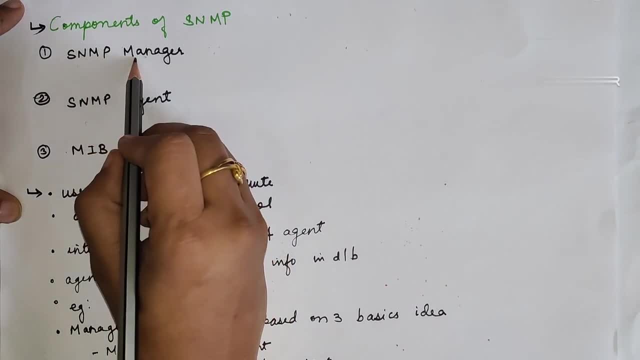 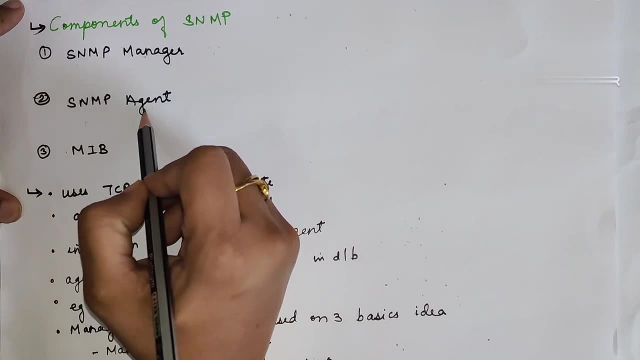 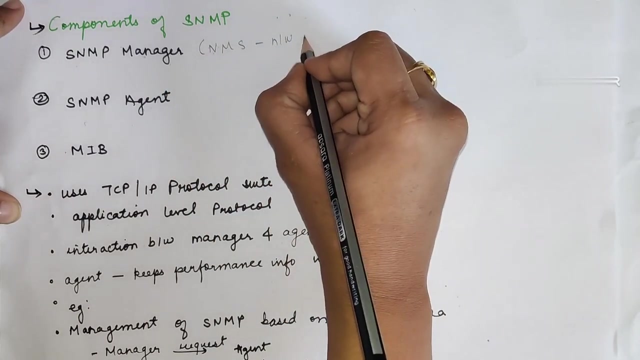 Now let's see one by one. what is that? We know what is SNMP manager. It is a centralized system used for monitoring the network with the help of SNMP agent. Sometime it is actually also called as NMS, that is, a network management system. 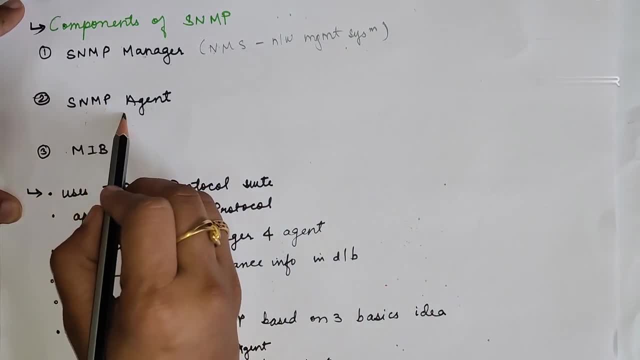 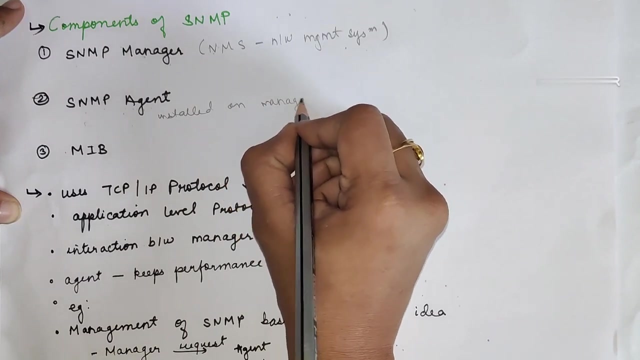 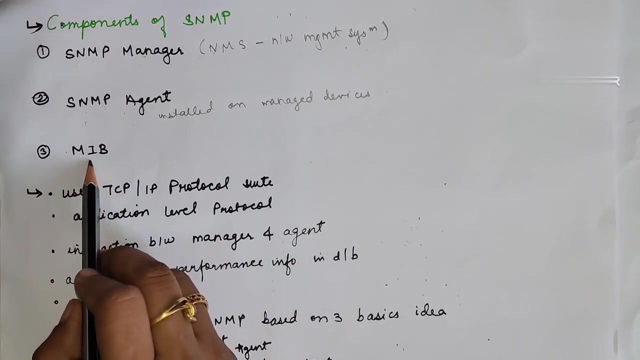 Now, what is an SNMP agent? SNMP agent is you can easily say that it is a software management software module That is actually installed on managed devices. This software is installed on that different devices. Now, what are this managed devices? This managed devices can be your PC. 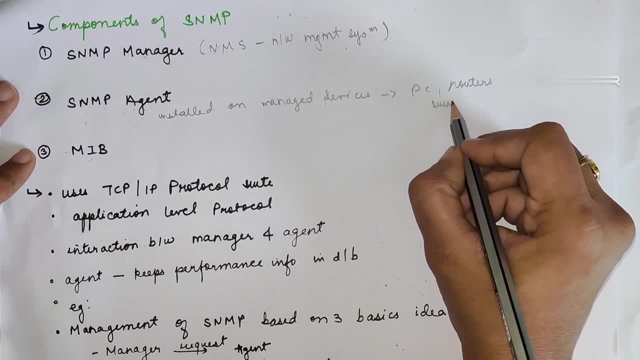 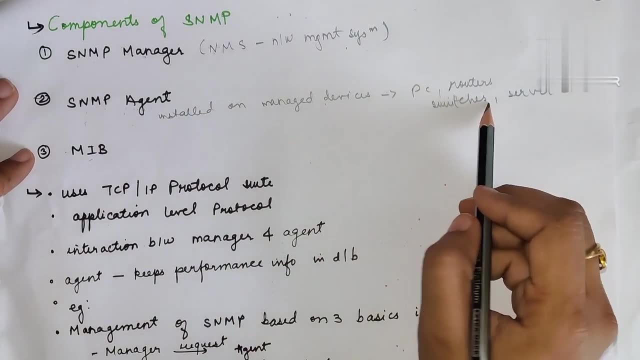 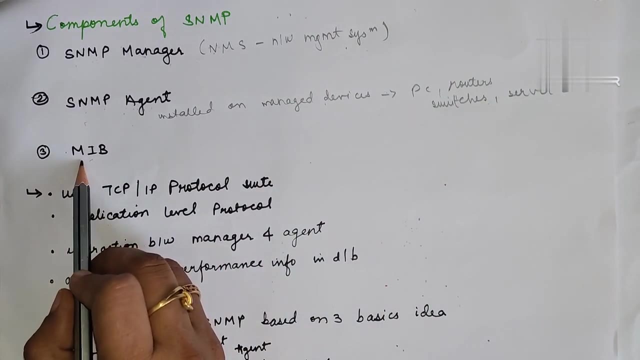 It can be your watch routers, it can be the switches, it can be the servers. so these are the different managed devices and this software module is installed on this devices so that it can track it very easily. now the third component that you don't know is an mib, that is, the management information base. 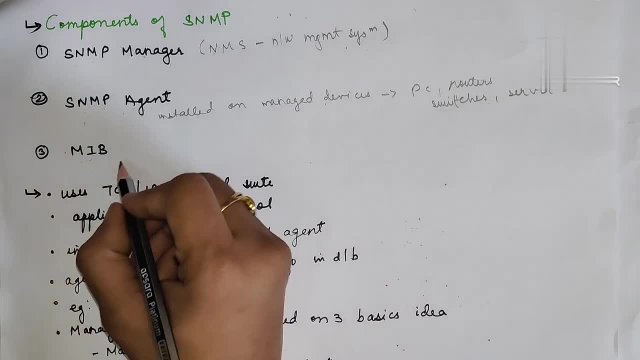 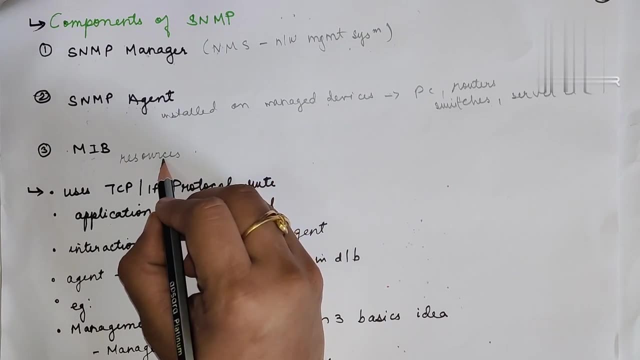 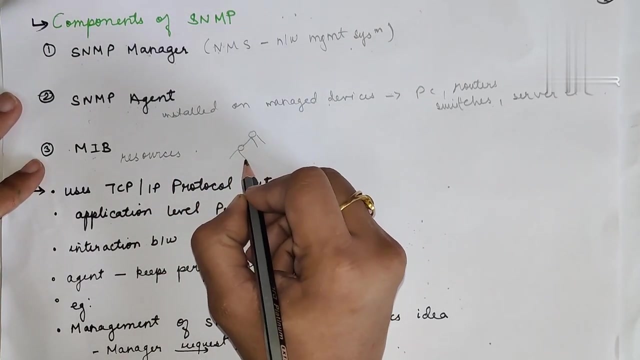 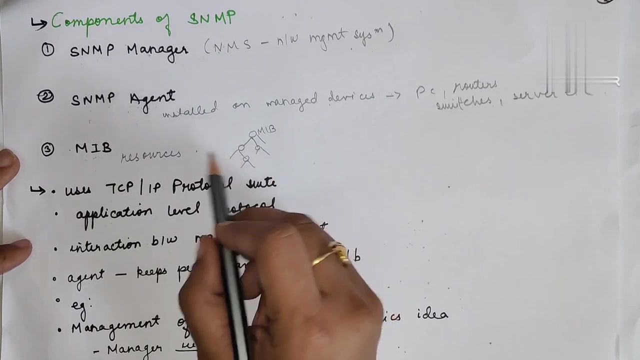 now why we require this. we require this to track about the resources, so it contains all the information that are required or used by this, resources, that are used for managing it, and it always uses hierarchical structure. in this way, it manages the information. you can say: this is mib and it uses or it organizes the. 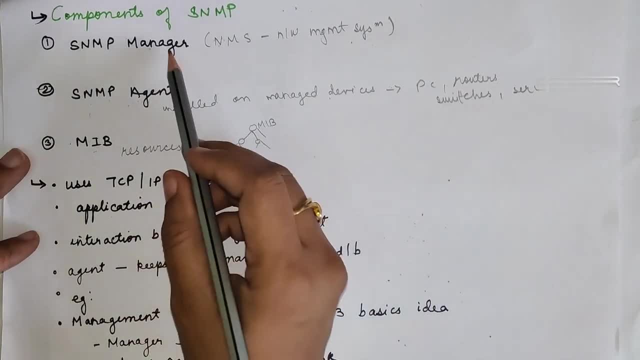 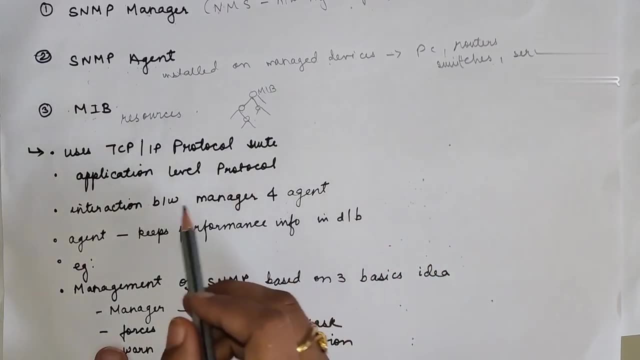 information in the form of hierarchy. now, these are the three main components that you should remember in an snmp. now, uh, there are some more important information that you should know about snmp. is that snmp is? it uses tcp, ip protocol suit and it is always going to work on the application level protocol. now you remember.